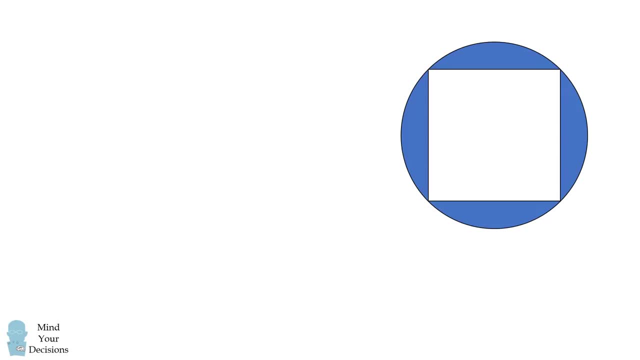 circle's radius. We'll do the same thing From the center of the circle. we'll draw the diameter that spans across the diagonal of the square. This has a length of 2 little r. The diameter of the circle is equal to the diagonal of the square. Therefore, 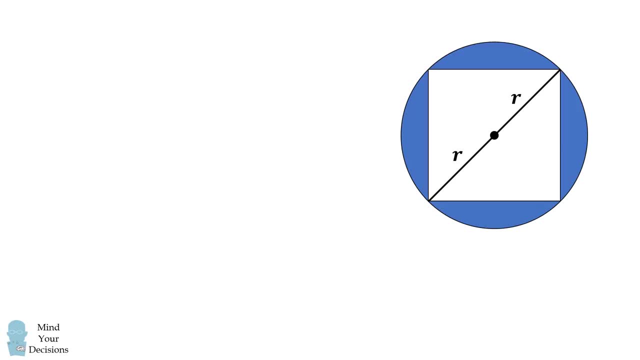 the side length of the square will be an isosceles right triangle whose height is equal to the diagonal of the square is 2r. The square's side length will be r times the square root of 2.. The blue area equals the area of the small circle minus the area of the small square. This 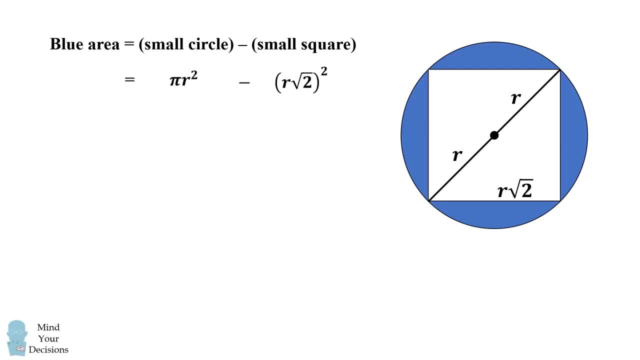 will be pi little r squared minus the quantity little r times the square root of 2 squared. This simplifies to be pi r squared minus 2r squared, which equals little r squared times the quantity pi minus 2.. We now know the blue area and 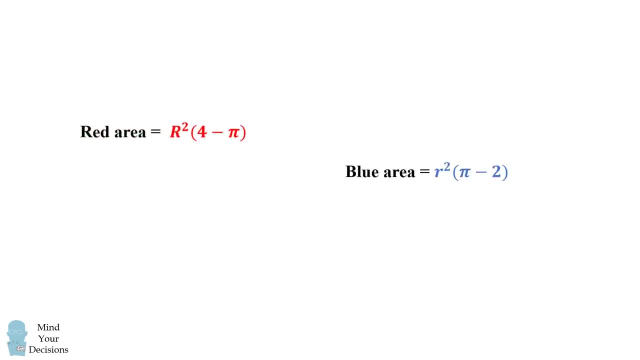 the red area. so we set these two areas equal to each other. We then take this equation and divide both sides by pi minus 4 and little r-squared. This gives us the ratio of the radii squared, and we then take the square root of each side. 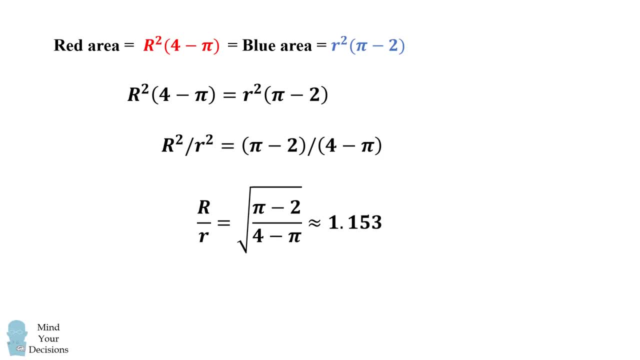 to get that the large circle's radius divided by the small circle's radius is equal to the square root of the quantity pi minus 2, all over 4 minus pi, And this is approximately 1.153.. Did you figure it out? Thanks for watching this video. 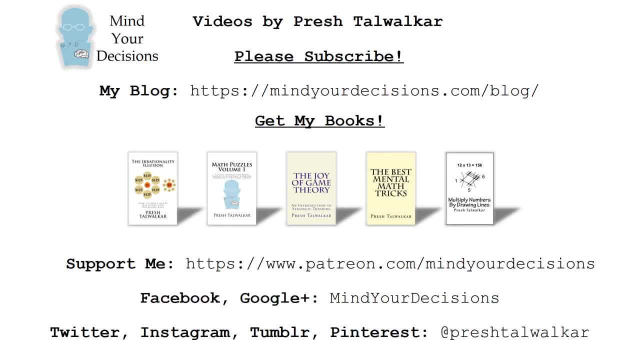 Please subscribe to my channel. I make videos on math. You can catch me on my blog Mind Your Decisions If you like this video. you can check out my books, which are listed in the video description, And you can also support me on Patreon. 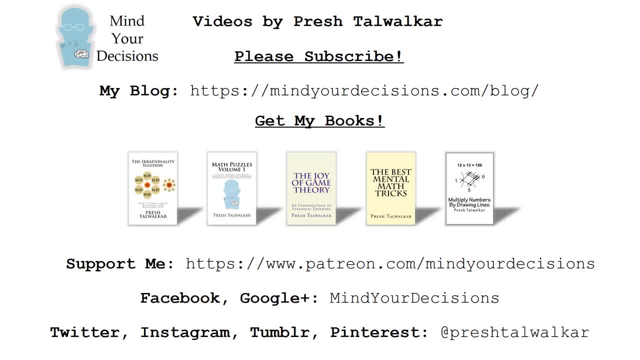 You can also follow me on social media, either at Mind Your Decisions or at Presh Talwalkar, depending on the site.